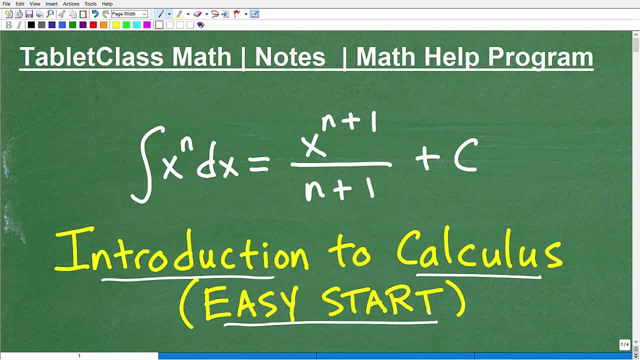 So, whether you're taking calculus or just have basic math skills, stick around for a few minutes and you'll be able to understand this stuff. Now, most people will look at this and they would just be extremely intimidating. They would be like calculus, Oh no, what's that? It's so advanced. You must be a genius if you understand this stuff And you know. I think it's natural to look at a bunch of symbology and be like I have no idea what's going on. 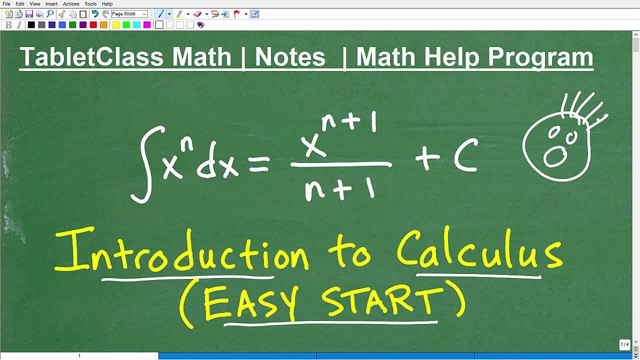 So, therefore, only smart people. Smart people can do this. Well, you know you can do this as well, because I'm sure you're smart. Okay, the whole thing is, you have to understand the language of mathematics, And we're going to try to demystify a little bit about calculus and show you a little bit of its practical usage, when calculus has infinitely many applications that are extremely important to our modern world. But, basically, I'm going to take this thing, which, look, can look a little intimidating, and explain it. 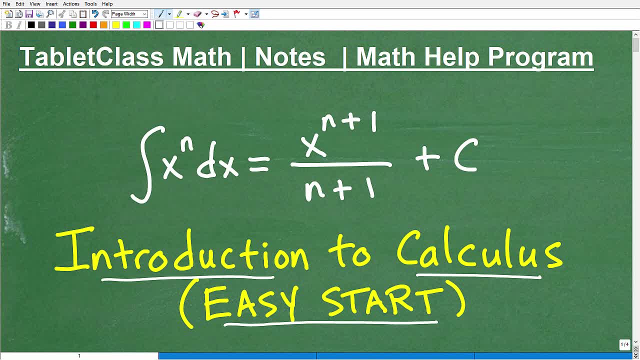 Anybody can understand here and and show you that calculus is not. it's not as bad as you might think. Now I don't want to minimize the challenge of taking calculus because it's a serious advanced mathematics and there's a lot to learn And you got to work really hard and you got to be really prepared to take calculus. So I'm not trying to minimize that. However, just for us to get a feel for the subject at a real basic level, we can definitely do that in a few minutes. So that's my 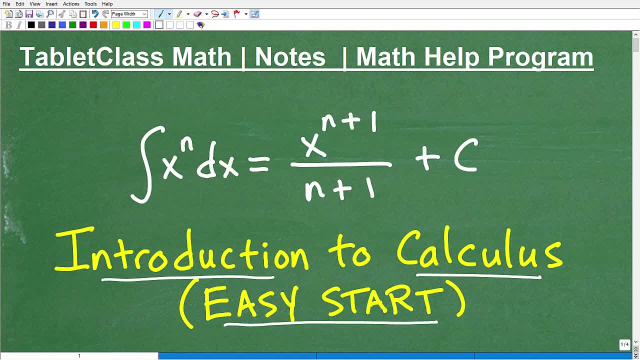 goal, And we'll see how I do if you stick with me for a few minutes. But first let me quickly introduce myself. My name is john. I'm the founder of tablet class math. I'm also a middle and high school math teacher And over several years I've constructed what I like to believe is one of the best online math help programs there is. of course, I'll let you be the judge of that. You can check out my math help program by following the link in the description of this video, But basically I have 100 plus math courses ranging from pre algebra. 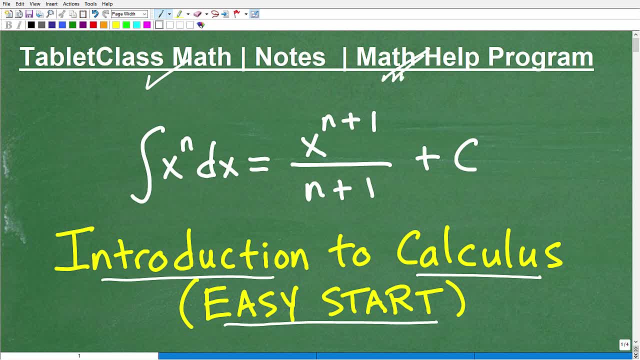 algebra one: geometry. algebra two: I'm going to be launching pre calculus here very shortly And of course that's the course you need to really learn in order to be ready for calculus And that's a pretty advanced math course. So again, we're just going to check out calculus here, But to be really ready for it, to take it out like at a college level, you do have to learn a tremendous amount of mathematics to be fully ready to study this subject. But we can certainly get a feel for it here in a second. 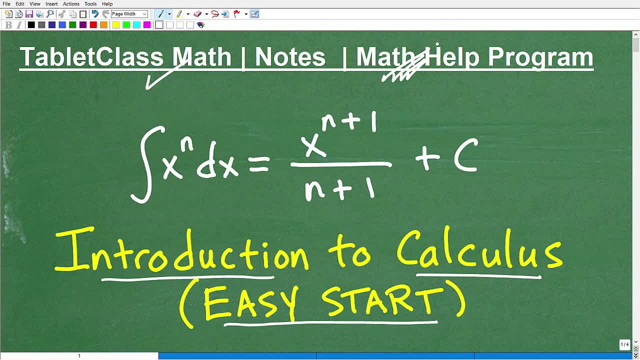 Also doing a lot in the area of test preparation. So if you're studying for the GED, SAT, high set, let's see here GRE, GMAT. I think I said those as VAB, acuplacer, Alex CLEP exam, teacher certification exam, nursing school entrance exam. there are a ton of exams out there that are very important for people's goals in life, that have a lot of mathematics on them, And if you don't get to the math section you don't do well on the exam. So if you are taking 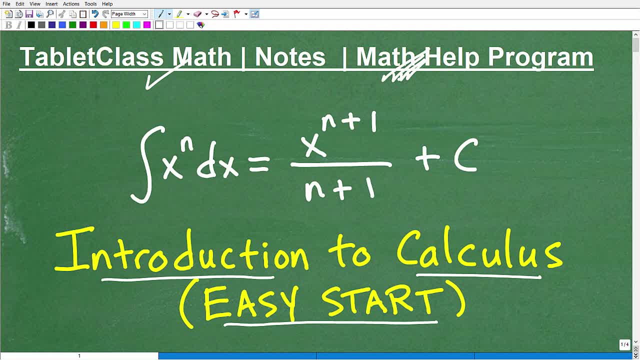 any one of these exams, go to my website, check out my full course catalog And I should have your exam. If I do not, please drop me a line And I will help you out the best I can. I also do a lot with independent learners like homeschoolers, been working with homeschoolers for years, have a great homeschool learning program And then, obviously, help those of you that are just struggling in your current math courses. Now, if you're truly serious about improving in math, you must do this, And that is note taking. So over decades of teaching mathematics, it's crystal clear to you. 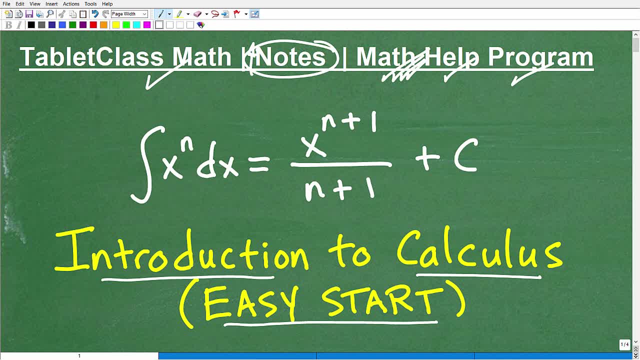 me that those students who take fantastic notes- I mean comprehensive, super great notes- they're going to do very, very well. It's almost a guarantee. And the reverse is true: Those students who like to talk to their friends, look at their cell phones or do their homework for other classes during math classes: well, you're going to have a tough time. And everyone always says to my: you know, they're like at this at the end of the year: why did I get a bad grade? Well, you got to hold yourself accountable, Okay. And 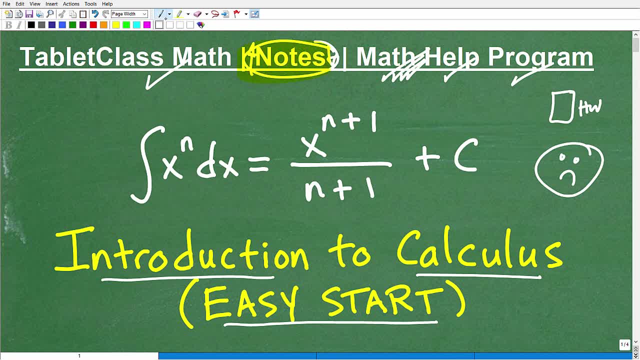 the one way to improve in mathematics- probably the foundational way- is note taking. you got to take great notes because note taking is focus. okay, they go hand in hand And the better you focus, the better you are focused, the better you're going to learn. It's common sense, But you know most people think that they can not focus or what. let's say this: that they don't have to write anything down and be focused. Remember, watching your teacher do math is not the same as 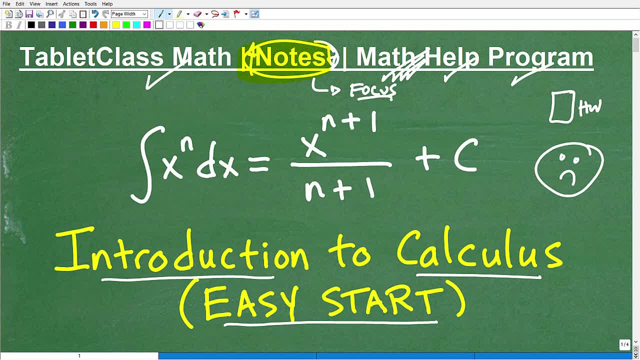 you being focused, you can. you can easily daydream And listen. I get it. I was a student once. I made all these mistakes and then some Okay. so you got to be focused And the best activity for that is note taking. By the way, if you need a great pair of notes- and you certainly do, because you need something to start from- I offer detailed, comprehensive math notes to include pre algebra, algebra one, geometry, algebra two and trigonometry. you can find the links to those notes in the description of this video. 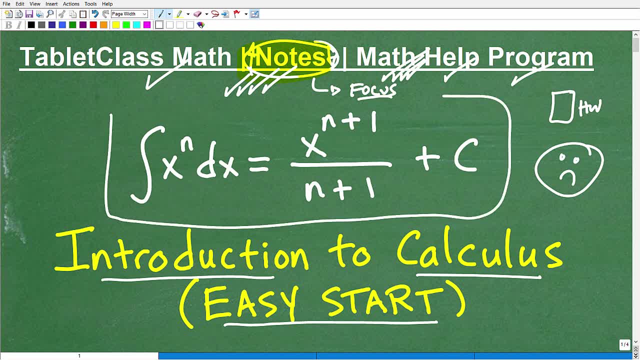 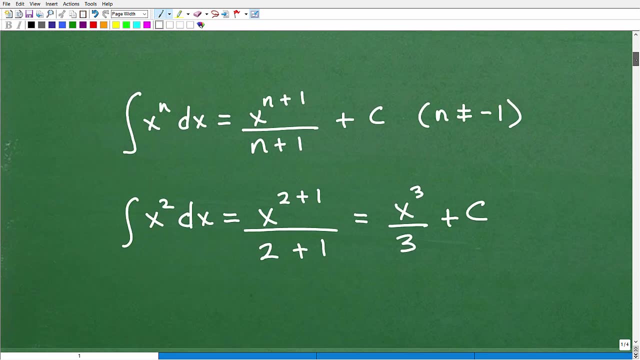 Okay, so let's get into this crazy stuff right here. And this is calculus, Okay, And this is one particular theorem. This thing right here is a special symbol, But let's explain this for a few minutes So you can walk away saying, Oh, okay, not too bad, All right. So this is pretty intimidating on its surface. Of course, if we don't even know what this is, you know we'll be totally lost, like anything. right, It's like a foreign language. Well, let's start with this thing. All right, this thing. 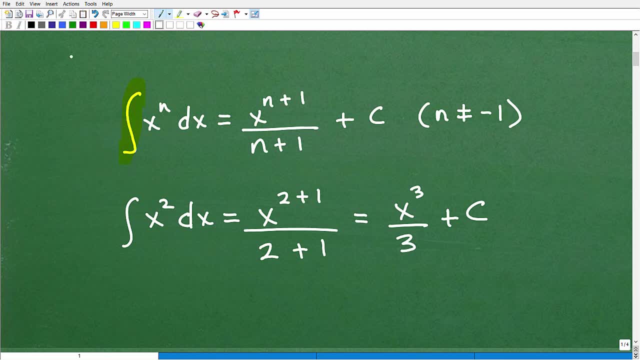 is called an integral Okay, and it kind of looks like a stretched out s. look like: right here we have an s And if we stretch it out, you know, kind of looks something like a stretched out set s. And, matter of fact, that's a good way to think about it, Because this is often referred to as elongated s And s is for some Okay. So some like: what are we doing here? Some of what? Well, we're going to be adding things up, And this symbol here is 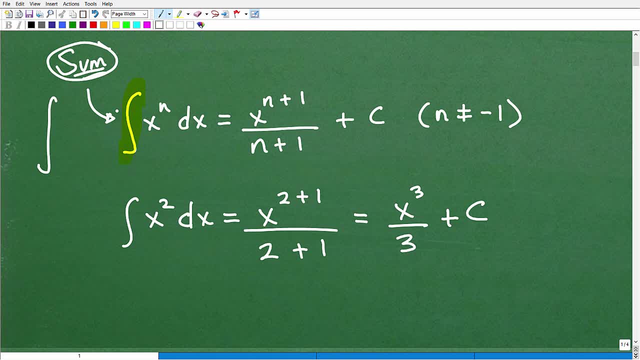 actually kind of a command or it's telling us: okay, add, add stuff up, add some stuff up, And it's called an integral. Okay, So this particular integral right here, this is technically we call this an indefinite integral. Okay, And now you're saying, well, what's this, all this mumbo jumbo mean? Well, I'm gonna explain this, because we're going to do a practical problem here in a second. So in calculus we're given rules, okay, a bunch of rules. In mathematics you get all kinds of rules. 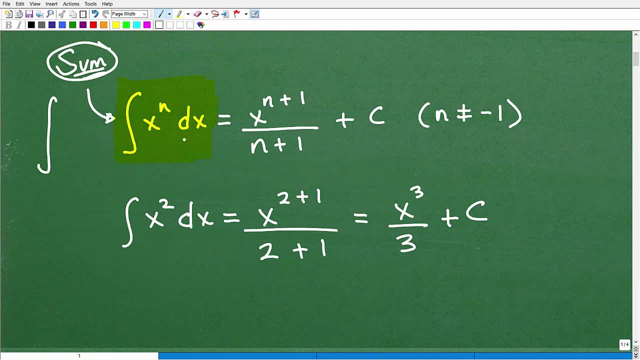 So we're saying the integral of x to the n power dx. don't worry about this little dx here. I'm not saying it's not important, but let's not worry about it now. But all you do, if you have, if you want to find the integral of x to the n- that's something to the n power, we just follow this little recipe. Okay, we go x and then we have an n here. So we're going to write an n plus one. Okay, we're just going to add a one to that, And then we're going to divide that whole thing by n plus one, And then this little plus c. 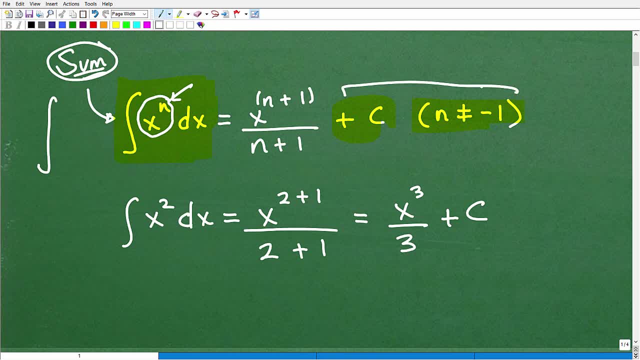 and all this little stuff. we can kind of disregard this for now, Not that it's not important. I know some of you out there might be taking calculus. Oh no, that's the constant, Listen. yeah, well, we can kind of minimize that for right now. Okay, we'll just kind of keep it simple. Now let's let's actually find the integral of something here. Okay, Now, even if you haven't studied algebra, just stick with me. Okay, Let's find the integral of x squared. 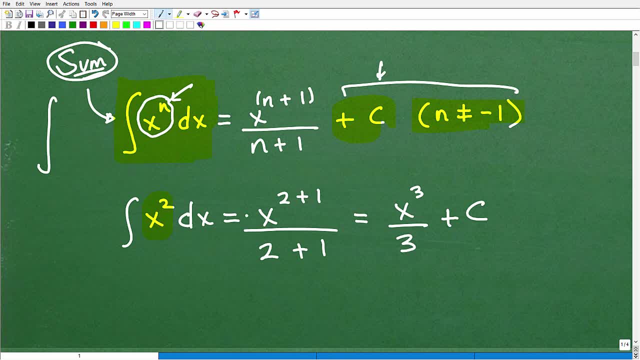 So let's follow the rule. Okay, x squared, So x squared. Okay, remember, the rule says: take that power two, and we're going to add one to that power. That's what that rule is right. So two plus one, All right. so x to the two plus one, And then we're going to divide by n plus one, which is that power plus one. Okay, so that would be two plus one. So we're just following the rule. So if you can follow, 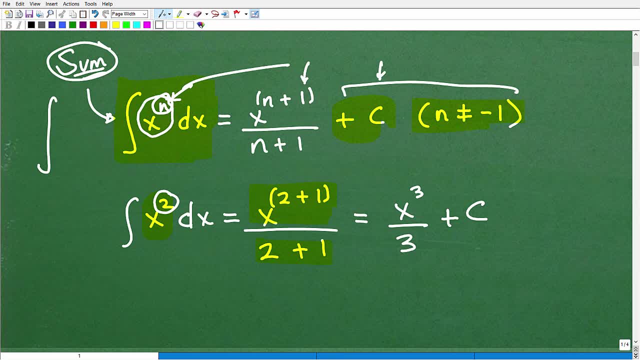 recipes. okay, if you go into the kitchen and you make something, you can pull up your recipe book and you can. you know you, I'm sure. if you make pancakes or something like that and you go to the pancake box, okay, or mashed potatoes, or whatever the case is in today's day and age, it's not too complicated. But just you know, you're going to take some of this, take some of that, you're going to do this, And then we're going to do this, this and this and boom, you get what you have. This is no different. Okay, this is like a recipe book, an algorithm. 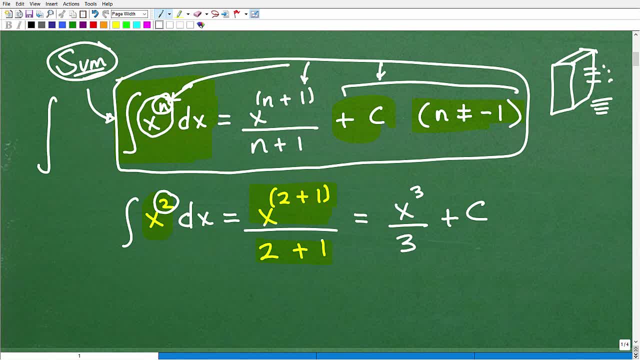 we call. there's fancy words for theorem, but basically it's a Hey, this is a rule, do this. it's a recipe. when you see this, we're going to do these steps, So let's simplify this. So x to. 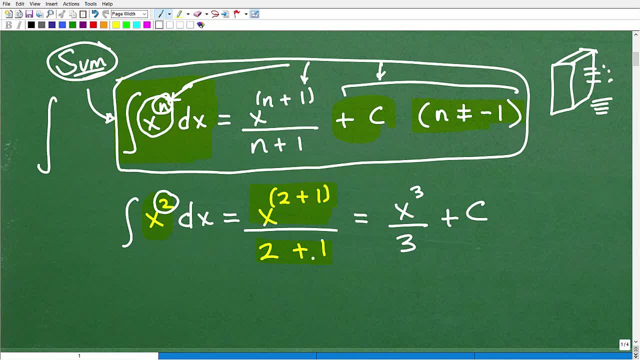 the two plus one is x to the third. power over two plus one is three. So the integral of x squared dx is equal to this. Now again, I'm definitely, you know, overlooking some things that are very important, no doubt about it, But let's just kind of keep it. 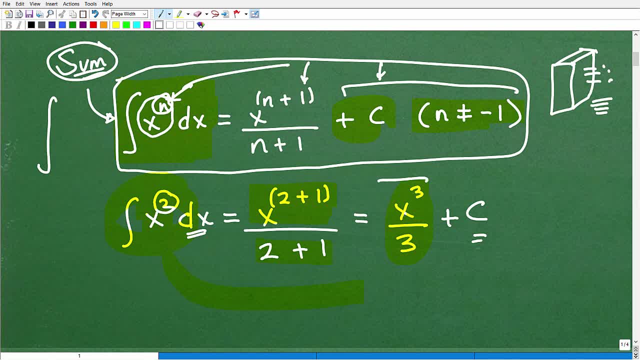 simple. Alright, so we have the integral of x squared dx is equal to x cubed over three, And so at this point, hopefully most of you can see how we went from here to here by following this rule. Very good, But what does this have to do with anything? And you might be saying to yourself. 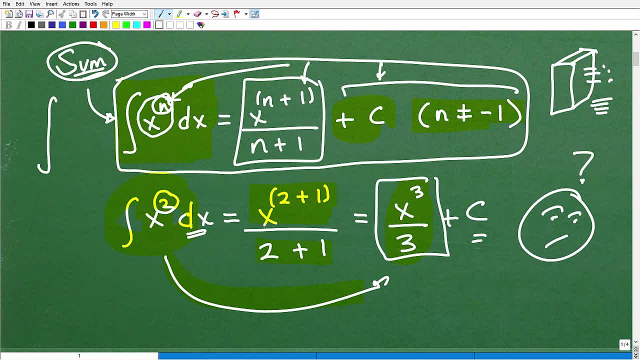 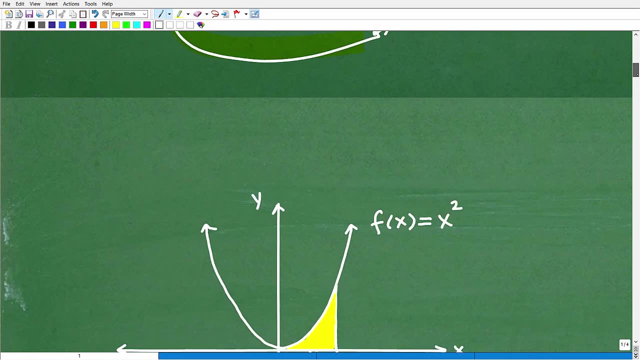 okay, I understand, But what's the whole application? What's the idea here? Well, we're going to go back to this concept of adding up and summing, So let's actually apply this in a real basic practical problem in calculus. Now, one of the videos that I've done: 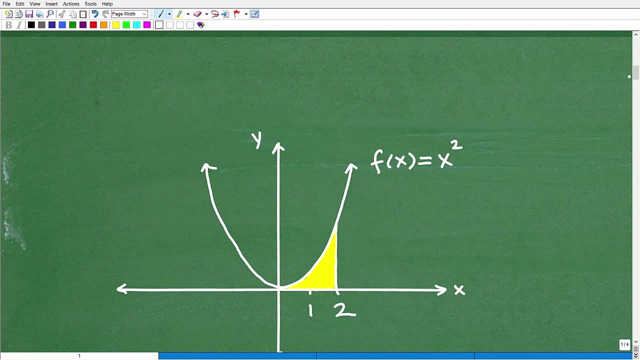 on my channel. matter of fact, I think it's the video that I have the most views with, And the last time I checked at least the time of this video, I think I had like 5.3 million views on this video And it was like understand calculus in 10 minutes And I kind of explained. 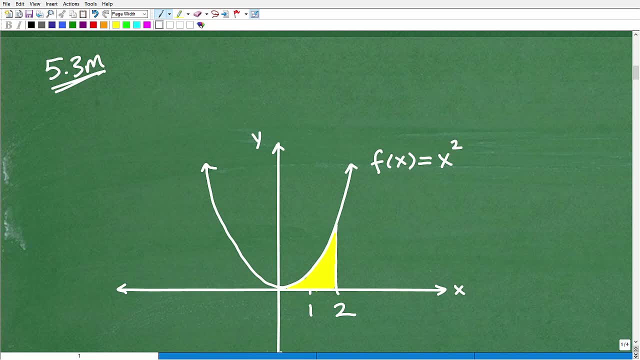 the real basics, essence of calculus and why we need it. And let me just quickly rehash this: Let's take a rectangle, Let's take a circle And let's take a triangle. Okay, So if I wanted to find the area of a rectangle, what would I do? Well, if I got the length and width, the area, 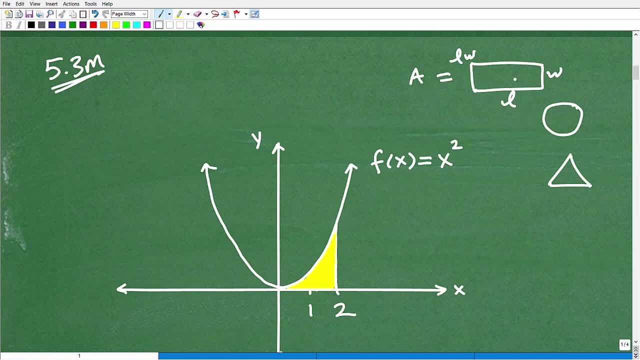 is equal to the length times the width. I have a nice formula, Okay, I could just follow. How about a circle? Well, the area of a circle is equal to pi r squared. And if you don't know that, the r is the radius, If I know the radius, I could follow this formula and find the area of that. 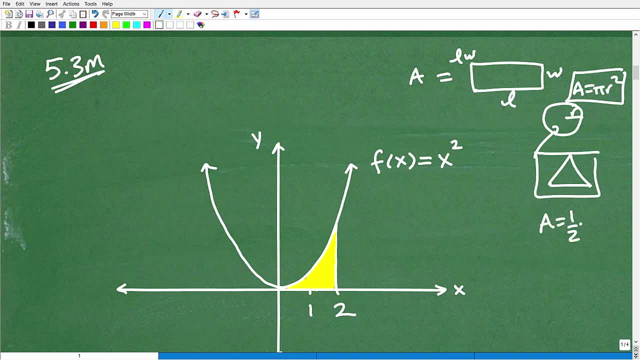 circle. How about a triangle? Well, triangle is equal to one half base times height. Here's the height, here's the base, And I can get the area for a rectangle, a circle, a triangle And there's some other basic figures. excuse me that I can get the area for, But how about the area for? 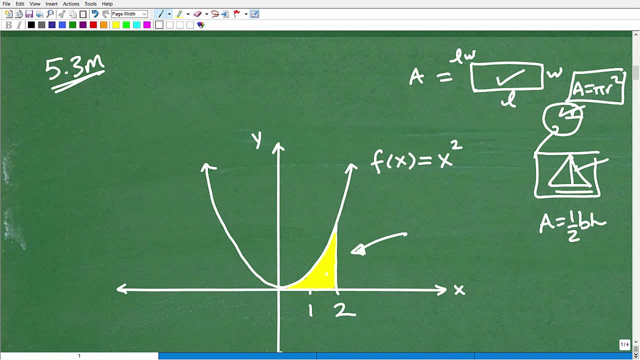 something crazy like this. Okay, so that little yellow part right here underneath this curve. excuse me if my voice is cracking up a little bit. This is kind of like allergy season for me, So I'm going to keep plowing away. 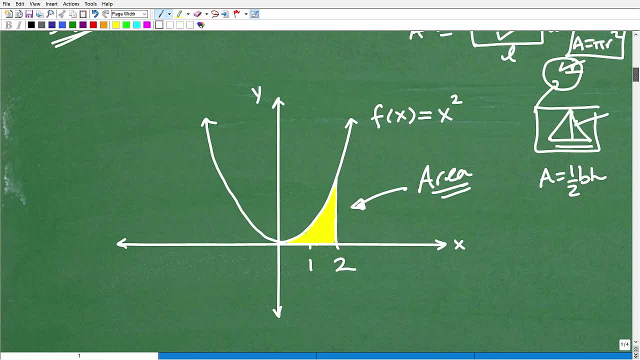 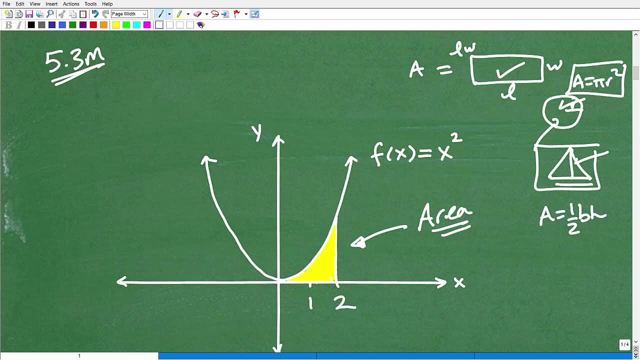 And hopefully this doesn't distract us for learning calculus. All right, let's continue to move forward here. All right, so what if I wanted to find the area of this little yellow sector right there? Okay, Is there a formula? Hey, give me a formula, I'll calculate. 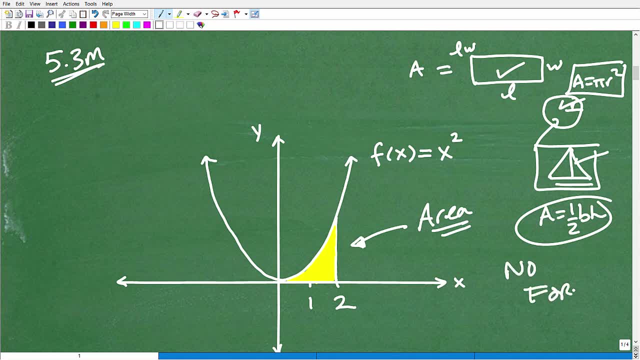 the area. Guess what? No formula, There's no formula. All right, so you're like no formula. Well then, how do we find the area of that yellow sector? Well, we need our hero in mathematics, which would be calculus. We need calculus, right And calculus. 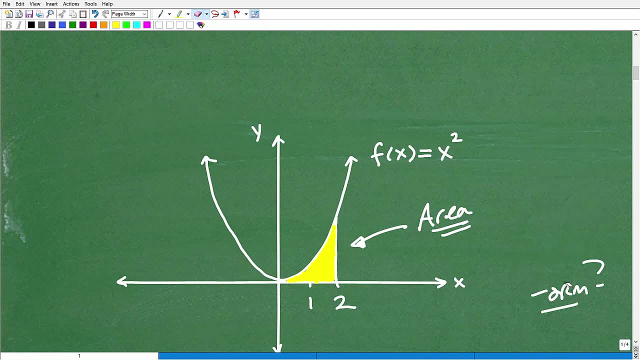 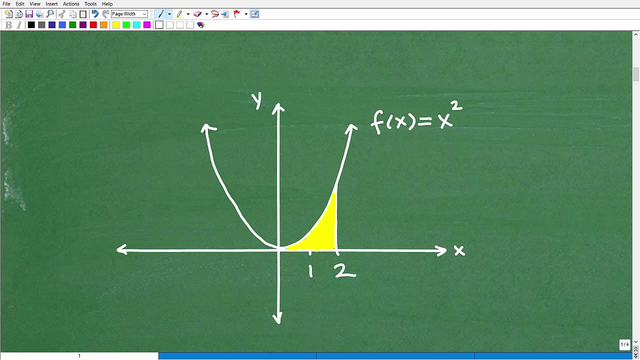 this is one of the main problems that calculus solves for us- is finding the area of all kinds of crazy, unusual shapes that we don't have a formula for. Now let's continue on here. Now let's look at this white curve right here. Okay, this, if you didn't happen to know. 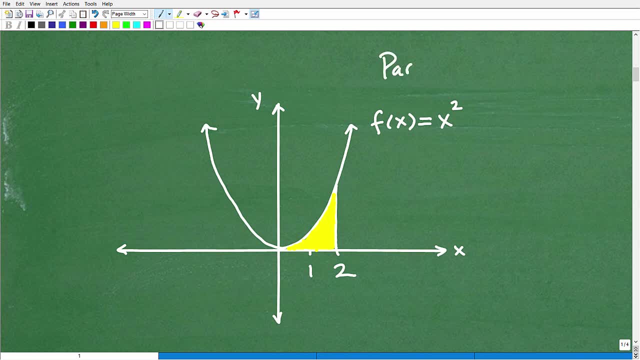 this thing, this thing right here is called a parabola. Okay, parabola, All right, and we describe it mathematically as this f of x is equal to x squared. This little x squared is a description of this shape. Okay, And what I could do if you're familiar with basic algebra. 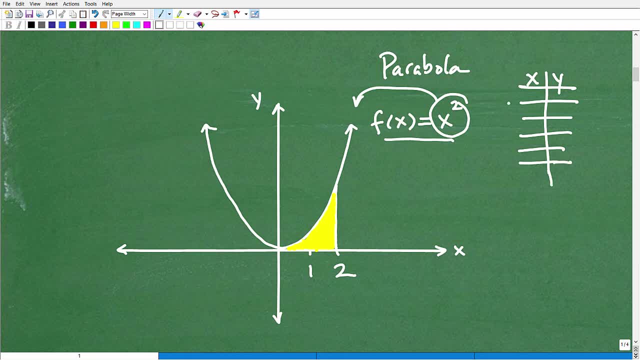 I can have a table right here And when I can just kind of say, okay, let's have some points. when x is equal to one, All right, I'm going to plug in this: f of x is the same thing as y. 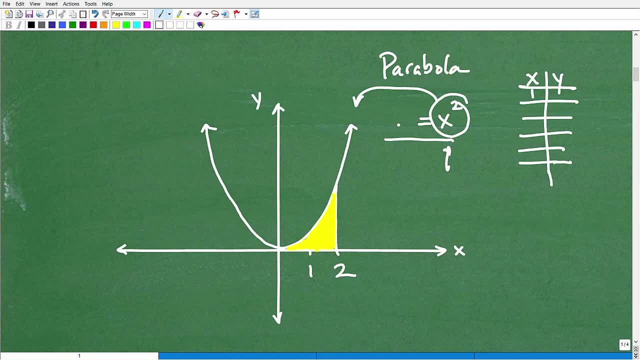 can just put this as y. Okay, so when x is equal to one, one squared y is equal to one. So the point one one is on this graph. Okay, right there. When x is equal to two, plug in a two for. 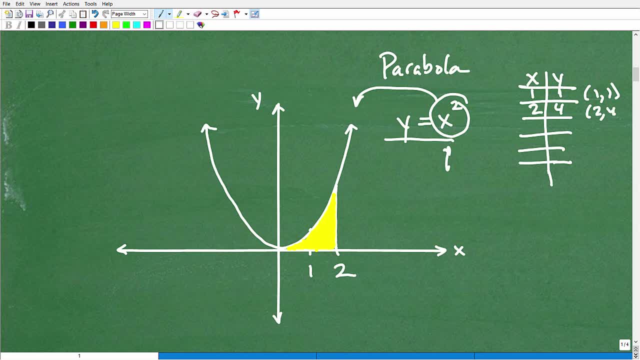 x, that's two, squared that's four. So the point two four is on the graph And we could just continue to make a bunch of points here to kind of plot this parabola down or plot this parabola on this x- y graph, But basically this little. 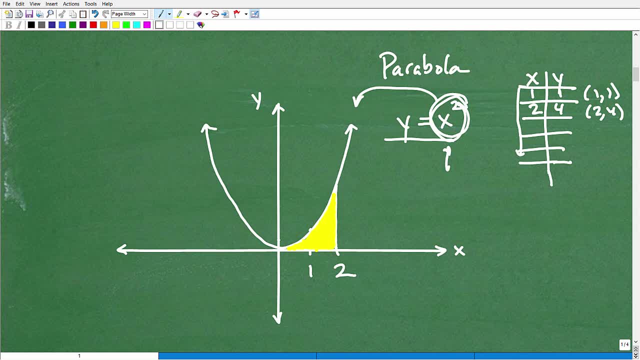 x squared describes this graph. Okay, now this y and this little f of x that I had, they're the same thing. y and f of x is the same notation. they mean a little bit. this is a function, this is an equation, But basically this y equals x squared. 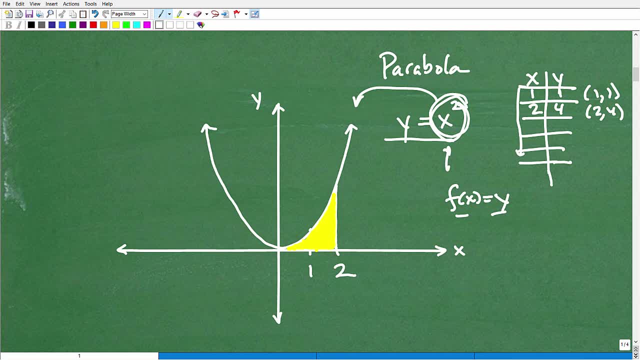 or f of x is equal to x squared, describes this graph right here. Now let's get back to finding the area underneath this curve. Okay, now it's bounded by the x axis, So that's a little piece right here. Well, this is what one of the great things for 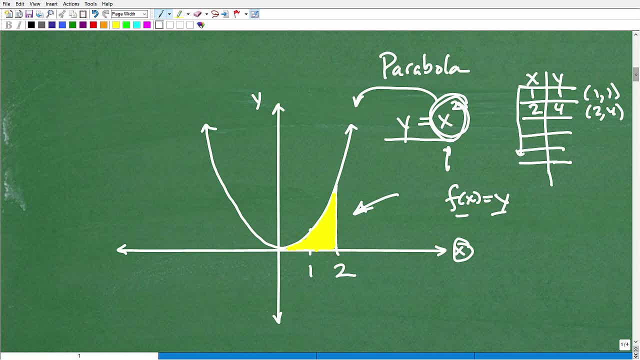 that calculus can help us with. So how do we do that? Well, what we're going to do is we're going to use that integral thing- Okay, that just showed you here- And remember that's the sum- and we're going to sum up all these little times, all the little, like real rectangle slivers. that. 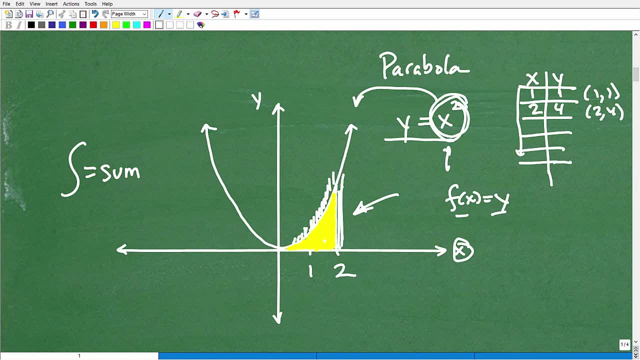 are underneath this curve, like right here. okay, we're going to under, we're going to add them up from zero, because that's where we're going to add them up from zero. So we're going to add them up to this, this starting that yellow yellow sector, all the way to two. Okay, so we're going to go from. 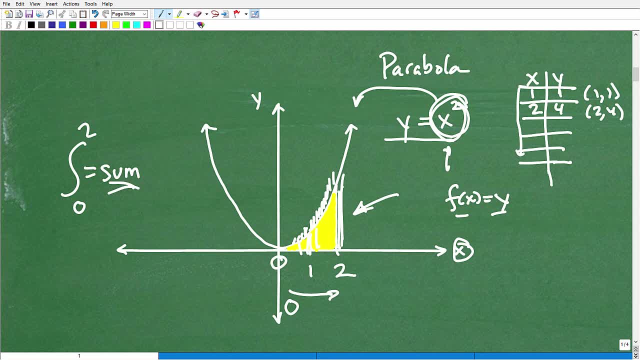 zero to two, We're going to add up all these little slices right in here underneath that curve, And if we add up all the infinite amount of the tiniest little rectangle slivers right there, we will get the area underneath that curve. So how does you know in a practical way? 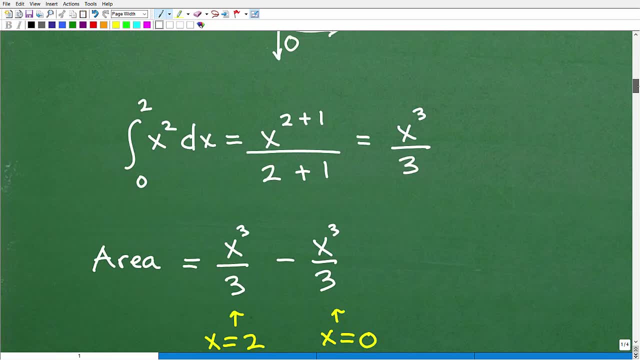 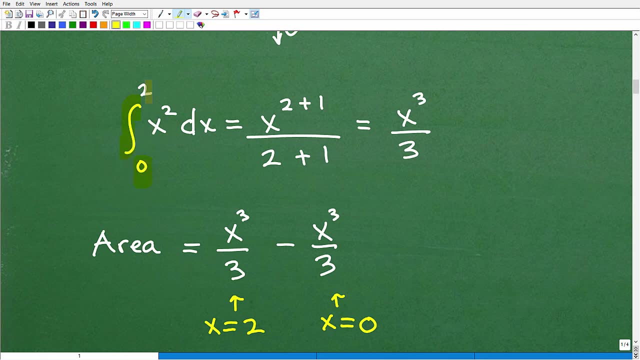 how does this work? Well, let's go ahead and show you now. Okay, So what we have here is an integral, Okay, and we're going to go from zero to two. this is called: we're basically starting from zero on the graph and we're going to end at two, right? So this is what this notation is saying. 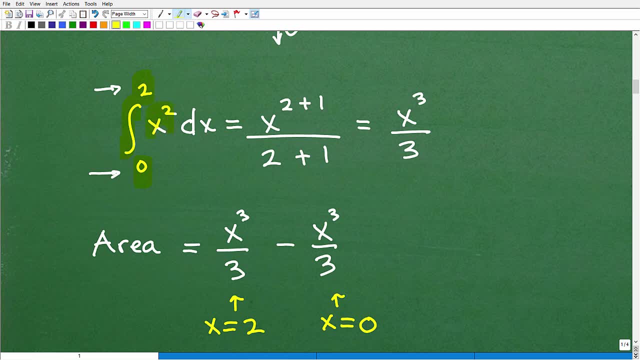 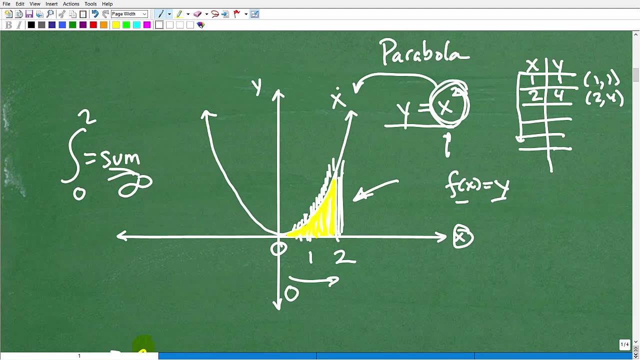 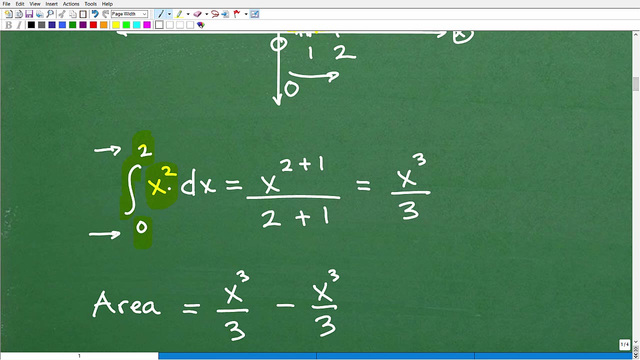 we're going to add up from zero to two And we're going to add up underneath that x squared graph. Okay, right here, this is the x squared graph, or equation: y equals x squared, But let's kind of keep it simplified. Okay, So from zero to two. 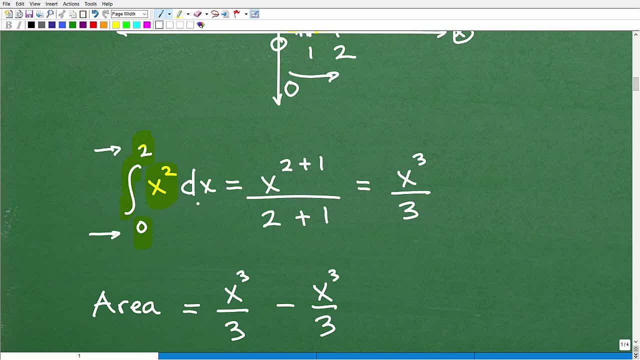 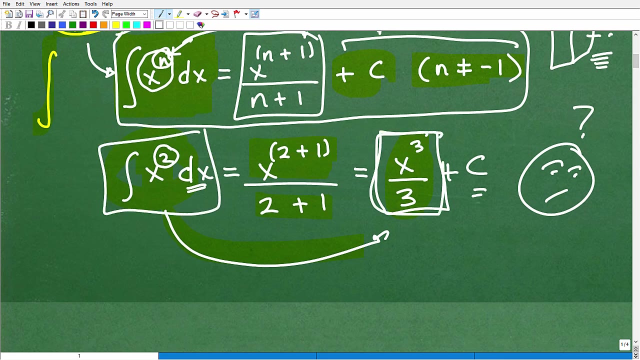 we're going to add up the curve underneath the x squared graph dx. that's just a little notation that we write Now. remember we just did this x squared. We just found the integral right up here of x squared, right. Remember we just did this problem. integral of x squared was equal to x. 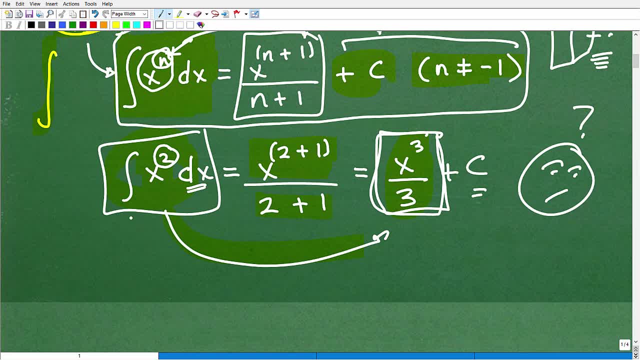 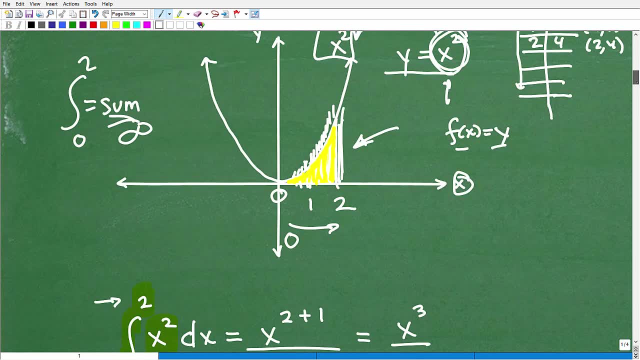 cubed over three. But in this problem we had no numbers here, we didn't have a zero, we didn't have a two. So this right here is called an indefinite integral And this one is called a definite, definite integral because we're now given values, all right, but we're going to do the same thing. 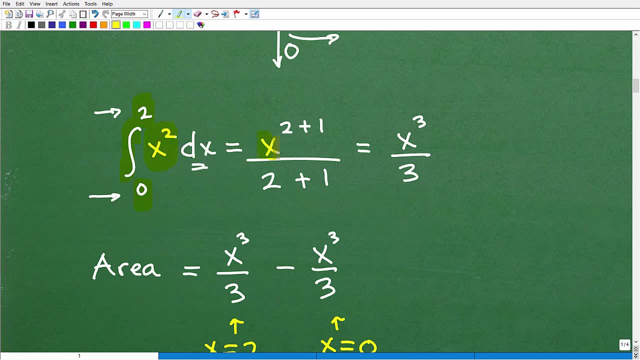 we're going to follow the same rule: x squared, uh. so we're going to remember: take our x at one to the power. okay, then we have. we're going to divide by that power two plus one. so this is what we got, and i explain that uh initially in our problem way up here. let's just quickly uh review. 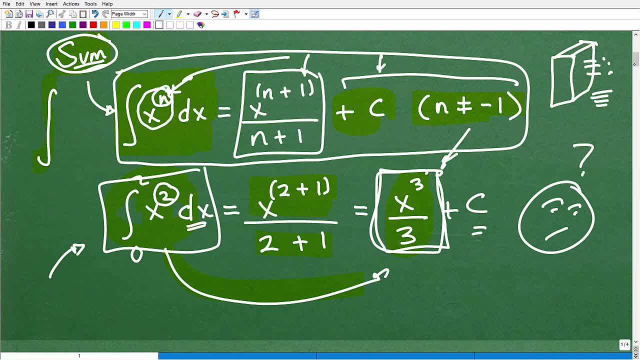 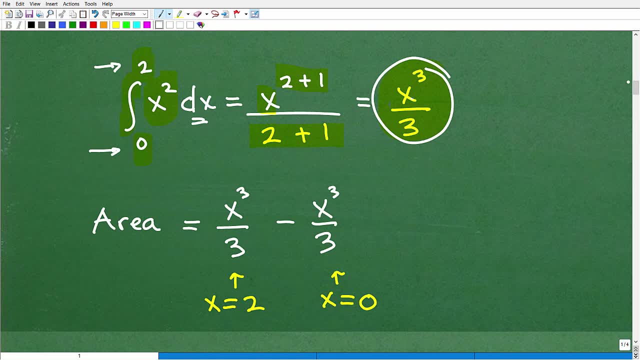 that we use this rule right here to get to that answer. okay, but now we're doing something with this. okay, but for the last, when i first uh introduced that, we were like: what are we doing with it? well, now we're going to actually do something with it. we're going to actually 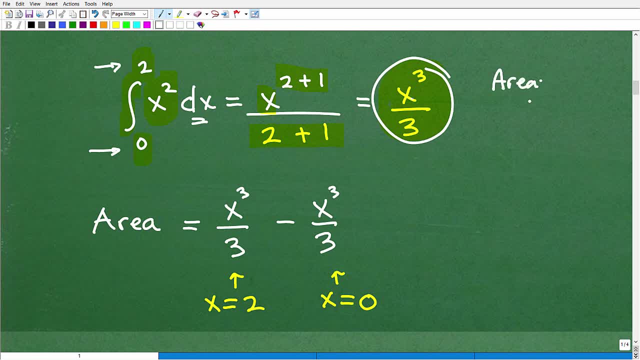 calculate the area. okay, we're going to calculate the area under the x squared graph. okay, from zero to two. okay, that's what we're, that's what this is telling us. hey, go calculate that area underneath the x squared function or graph, between zero, starting from zero, ending at two. all right, so. 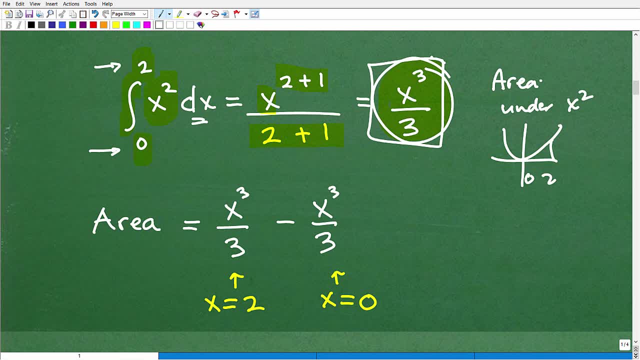 we have to use this and now, uh, we can, we need to, uh, excuse me, uh, calculate, uh with this um x cubed over three. now, how do we find the actual area? well, what we're going to do is take this x cubed over three, we're. 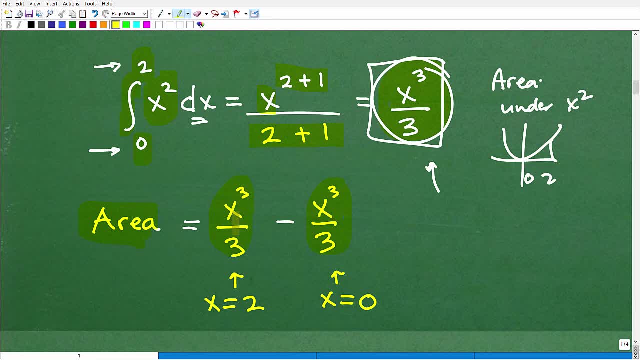 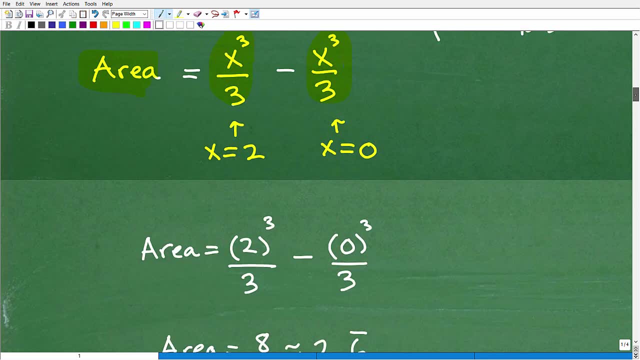 going to subtract it by itself: x cubed over uh, x cubed over three minus x cubed over three. we're going to subtract it by itself, but not really. we're going to add in particular values. so remember, from here on our integral, we have from: 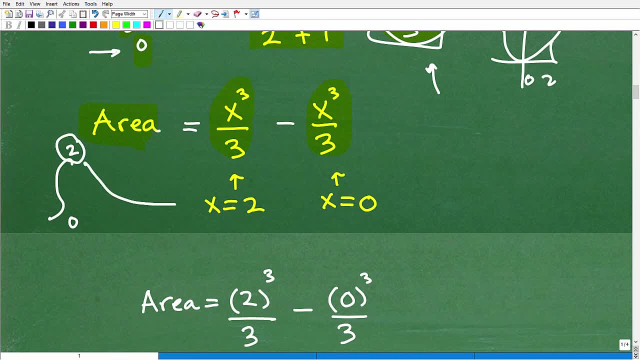 zero to two. well, we're gonna this two value. we're gonna let x equals two, right there, okay. and this zero value, we're gonna substitute in for x a zero from right here, okay. so when you have your integral, okay, this top number, right here, we're going to substitute in this x for that top number and then 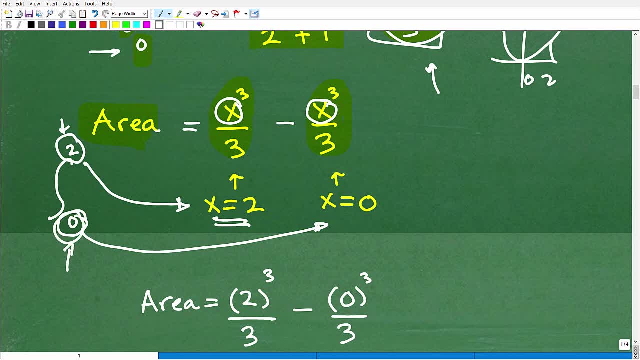 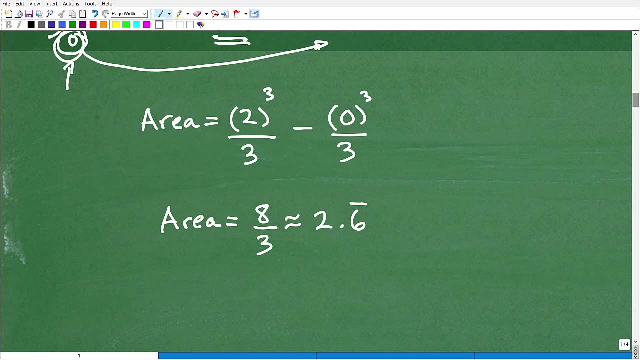 this x right here, we're going to substitute in this bottom number. okay, that's all we do. you do this in every single integral problem, so let's go ahead and do that now. so to find the area. remember we had x cubed over three and we're. 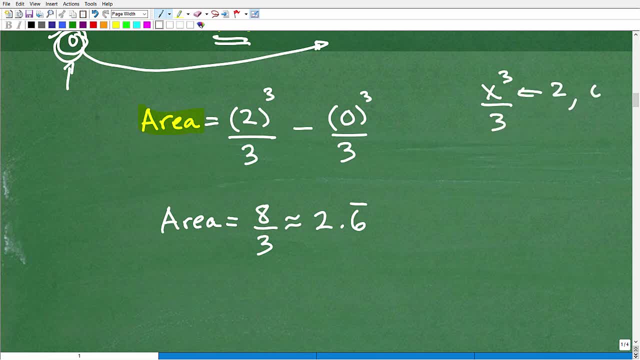 going to replace this x with the two, and then we're going to replace it with the zero. so first let's use two. okay, that's what comes first. so that's two cubed over three, and then we're going to subtract it from here is zero. okay, remember our second one. we're going to have that x equals. 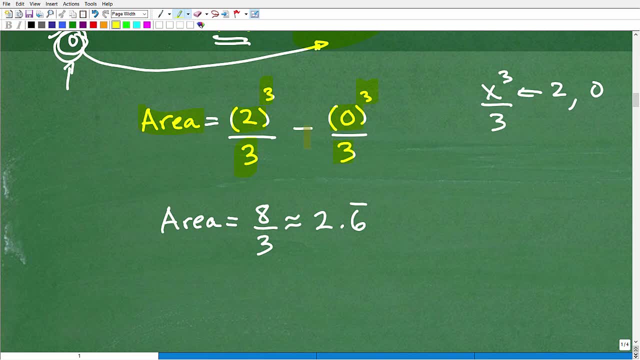 zero, zero cubed over three. and when we do this calculation right here, we'll get the actual area all right. so let's see how this goes. so two cubed is eight, two times two times two, so that's eight over three. uh, we're going to subtract away. zero cubed is zero, zero divided by three. this: 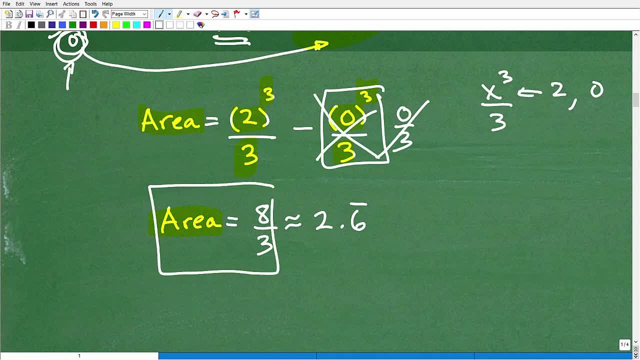 whole thing is zero. so we end up, the area is equal to a third, and if you go into eight thirds, if you go into your calculator, that's approximately, uh, the decimal 2.6 repeating, and that's it. we just found the area underneath this curve right here. 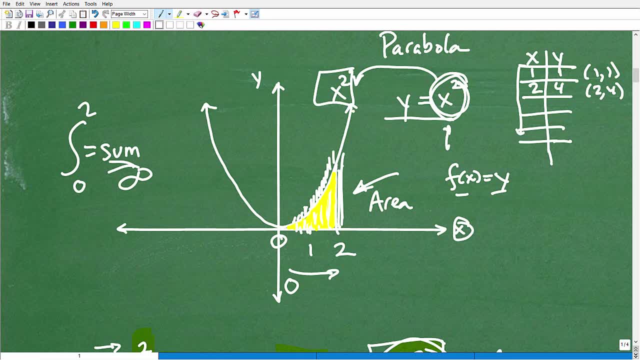 okay. and uh, let's say we wanted to go all the way out to three. okay, and find that area right here, well, but what you know? or actually, let's even make it better. let's say we wanted to go from- let me use a different color. let's say we wanted to go from one to three, this part right here. one to three- what? 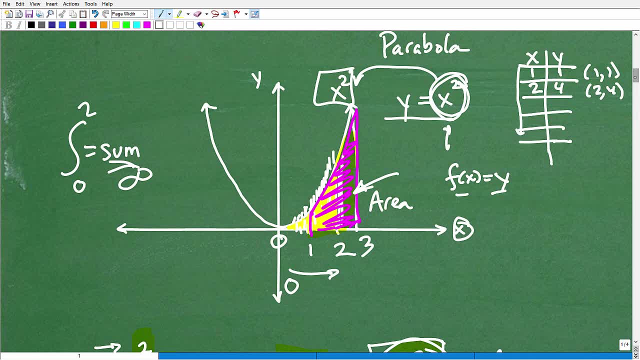 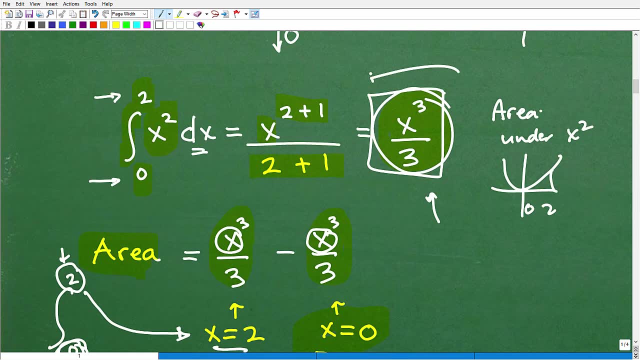 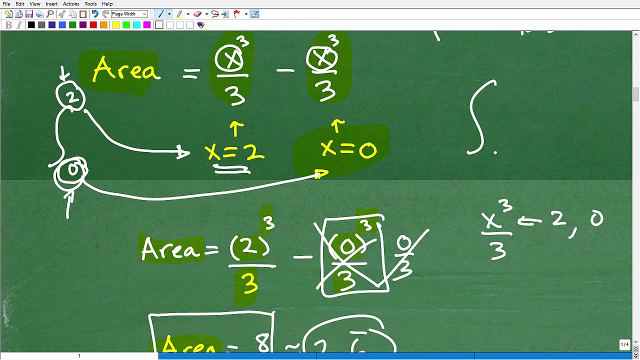 would we do? well, what we would do is take our integral and start it from one and end at three. okay, so we would do this same uh, this. we would still use this right here. but when we went to go evaluate, right, uh, at this point, okay, we would evaluate from one to three. we would plug in a three for this first one and a one right here. 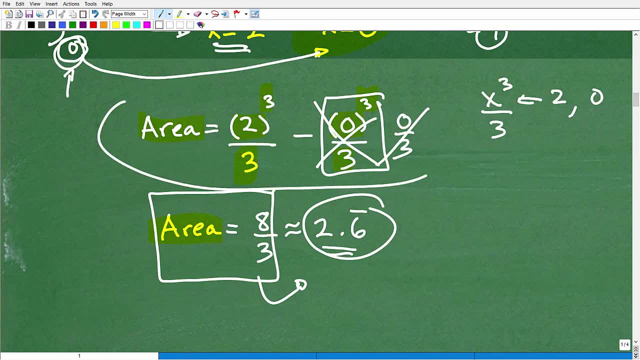 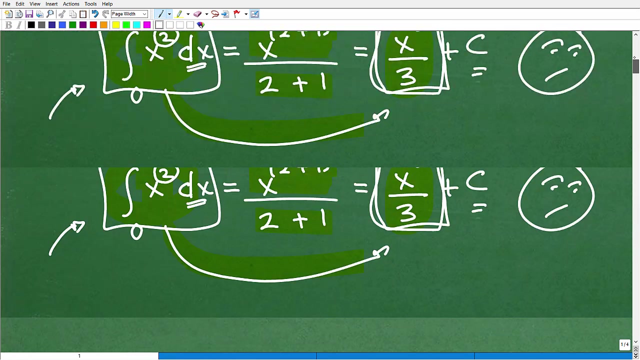 and do the math, just like as we did right here: all this calculation and we would find the area of the underneath that uh curve between one and three, so you can start seeing how powerful calculus is. and not only that, we can find the volume, all kinds of crazy shapes, and it's this. it's a fascinating subject and I hope I did a decent job. 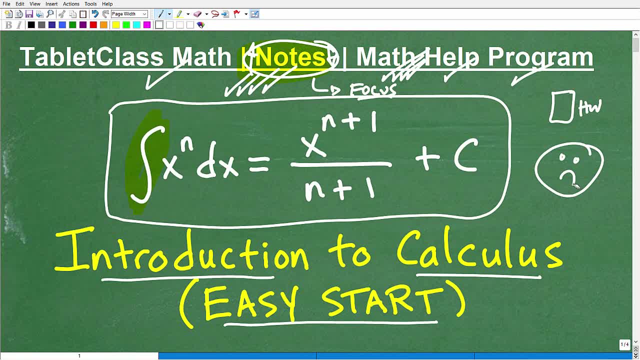 introducing you to the concept of calculus. okay, because I want you to take it. you know, I want you to actually study this one day and I've had so many people through the years in my math help program just start getting interested in mathematics. it started with algebra one. I'm like 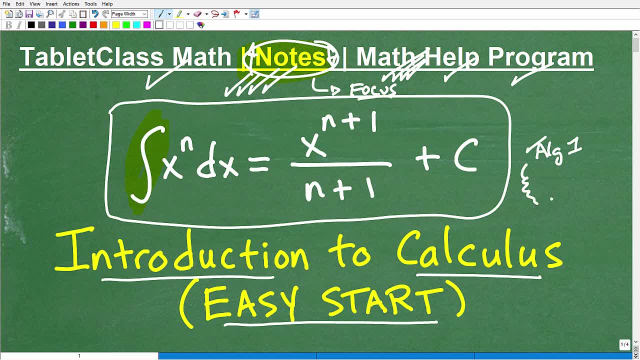 you know what I'm pretty good at, math I'm interested in, and they worked their way all the way up to taking calculus, okay, and calculus, again, it's such a fascinating subject, it's, it's, uh, the applications are infinite, okay, and all our modern world, so many of the things that, uh, you know the problems that. 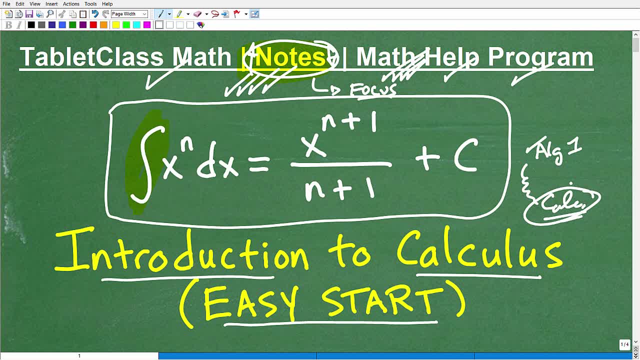 we have to solve. the technical problems that we have to solve involve calculus, but you can learn as well. okay, it just takes motivation and, hopefully, interest. okay, and if I've done my job with this video, despite my crackling voice- uh, you know- then you know, hopefully I've motivated you to at least 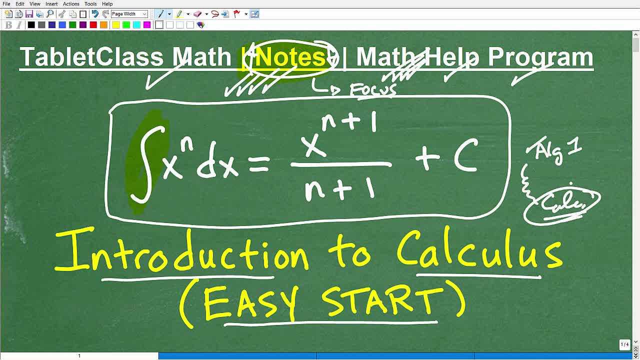 you know, consider, you know, working your way up towards taking calculus. you don't have to do it all in one shot, but if you do take calculus in an actual, let's say, college, I don't offer calculus because I think it's one of those subjects that you should take in a college classroom, but I do um. 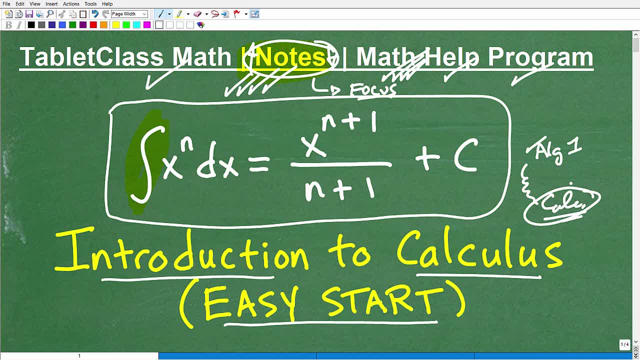 I am going to be launching my pre-calculus course here, which is pretty advanced mathematics for sure. okay, you have to be ready for this, because this is a real kind of basic concept of calculus. yeah, it gets much more sophisticated beyond this, but if you understand this, you just take. you take any subject, one you know, one little thing at a time. okay, all.